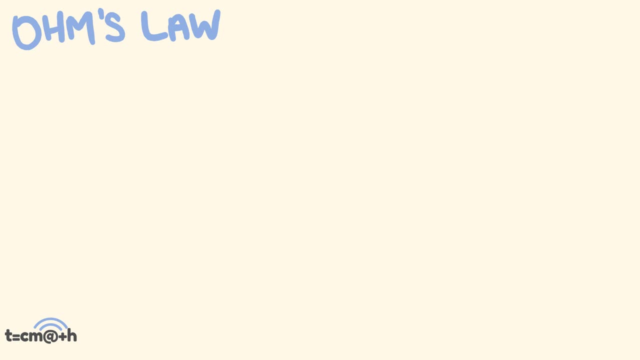 is not going to take too long. So, before we get to Ohm's Law, I'm just going to quickly show you an electrical circuit and how Ohm's Law relates to this. An electrical circuit, you know one of these. it's where we have a power source, such as a power point or a battery, as we have here. 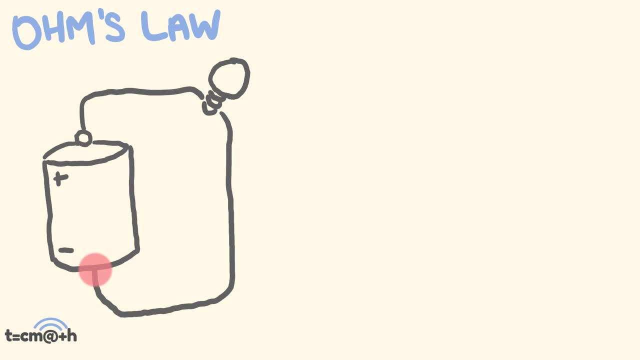 We have a bunch of wires coming from it, and then we have some fun item that we're trying to run, such as a light or a fan, you know, stuff that you plug into power points or need a battery for The first thing we're going to consider is this part here, which is the power source. Now a power. 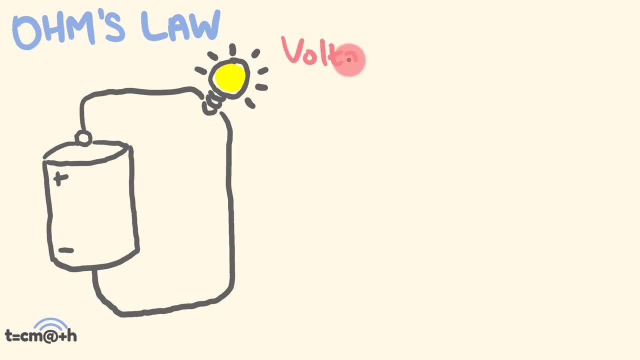 source- a battery or a power point- it provides the voltage, and when we talk about Ohm's Law we give this the letter V. Voltage is measured in volts, and they also have the unit of V there and pretty much what this is. it's the electrical potential between two points here. So 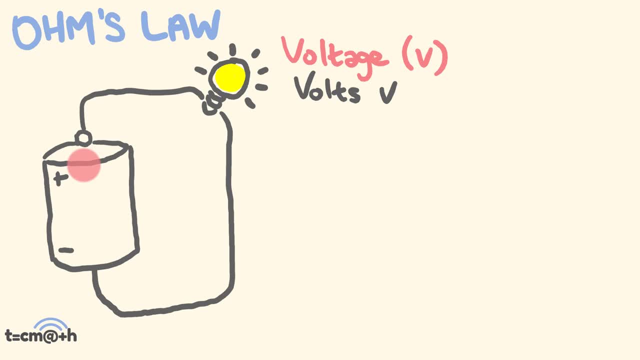 pretty much a nice way of saying the pressure of pushing electrons down a wire, But you can just think about this as being power. The second part that we have is the actual power that is running along the wires here, and I guess if we could actually have a look at this wire here, we could 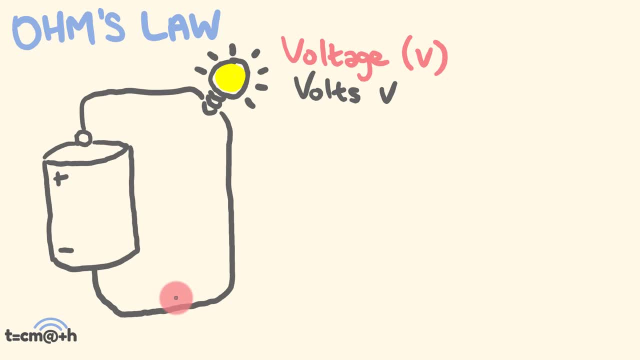 open it up and we could see how much electricity or how many electrons are running past a given point at a given amount of time. This flow rate, This flow rate is called the current, The current flow rate of electrons going past a particular point, and it's given the letter when we use Ohm's. 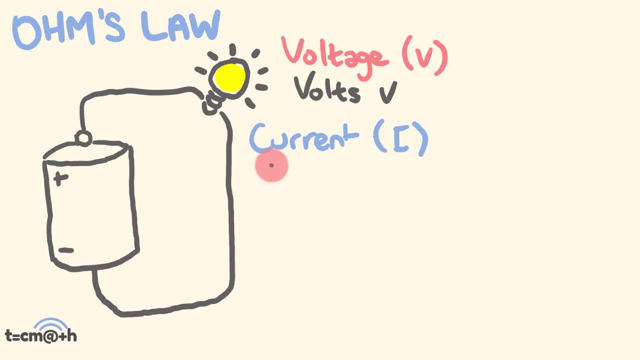 Law of I. We measure current in amps which have the letter A. Now look I. I think it might actually stand for intensity or something like this. I'm not 100% certain on that. one Don't know why they didn't give it the letter C. Maybe it's going to confuse people with a coulomb, but we use the. 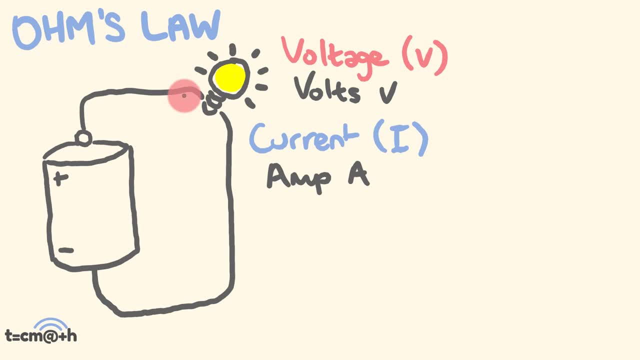 letter I for that. So current is the amount of electrons flowing down this wire. And first off, what Ohm's Law says is the following: It says that when we consider voltage and current, that voltage is directly proportional to the current. That is to say, if you were to increase. 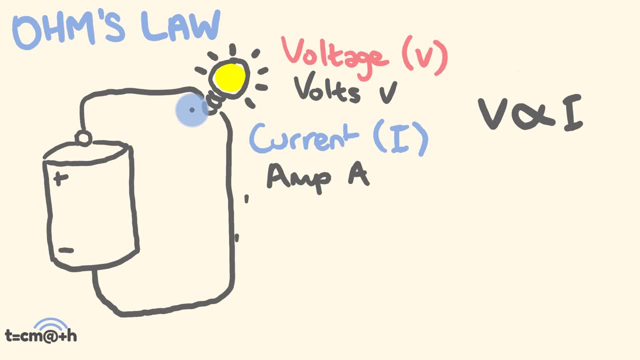 the voltage in this battery here, you would increase the current going along the wires there. And if you were to decrease the voltage of the battery here, you would decrease the current going along the wires. Now, these are not the only sets of numbers that we need to consider. 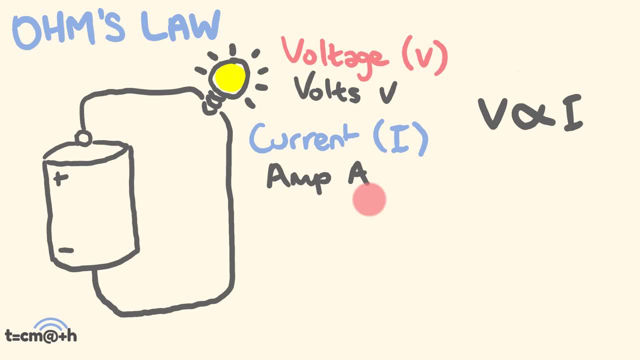 with Ohm's Law, There is one last set of numbers that we need to think about, And that is the resistance Which, when we talk about Ohm's Law, is given the letter R, And resistance is measured in ohms, which is given the Greek letter omega. Now resistance, if you imagine as electrons are. 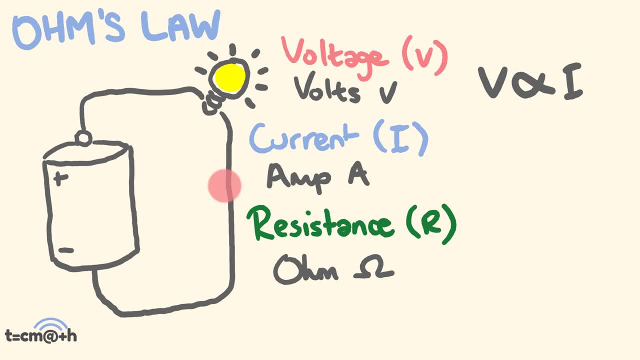 moving along this wire. they have all sorts of parts of the wire that are causing resistance. They're impeding the actual flow of electrons. It could be that they're made of a different material that has more ions on it that slow the electrons. 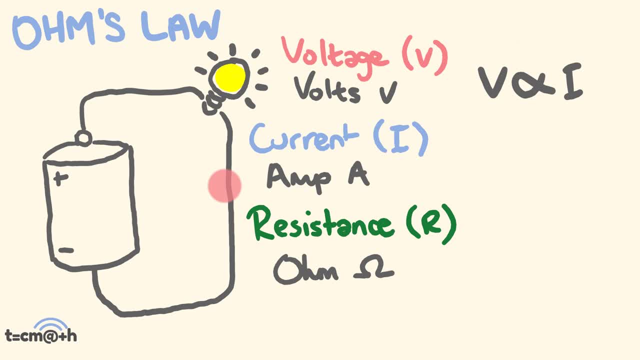 That's the kind of resistance that we're by the current. now, this is usually written a little bit differently and you might have seen this written depending on whether we're talking about voltage, current or resistance. we could change this all around and we could actually say, okay, what we have is we have the voltage. 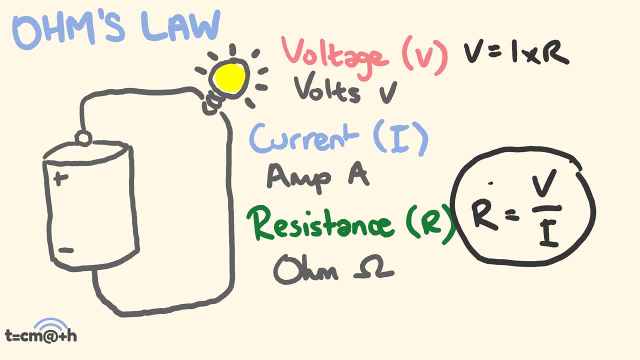 and that's equal to the current multiplied by the resistance. or we could also say that we have the current and that is equal to the voltage divided by the resistance, depending on how we ordered that particular equation. but just one little thing. there's a really, really easy way that we can. 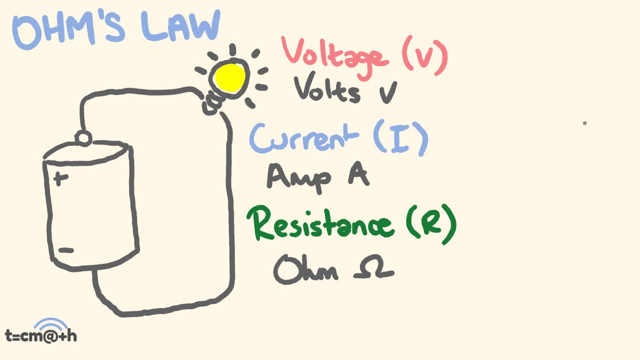 actually remember this, and i'm going to show you this right now. we can put all of these together in a triangle, known as the ohms law triangle, where we could say: voltage is equal to the current multiplied by the resistance. let me show you how this particular triangle here works. so, so we wanted. 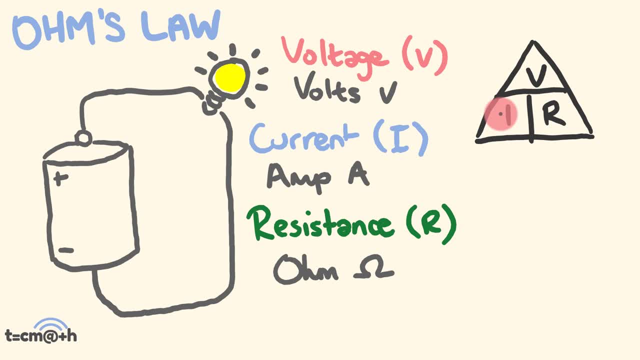 to work our voltage. here we put our finger over the voltage and, as you can see, current is sitting next to resistance here. it means we multiply these guys, so voltage is equal to current multiplied by resistance. so we will try to work out the current. i'll put my finger right here and i could say the current is equal to the. 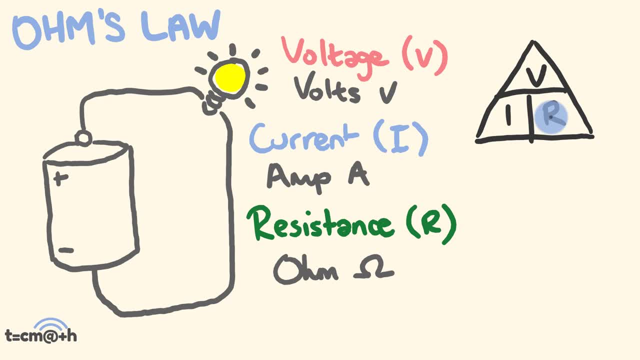 voltage over the resistance, voltage divided by the resistance. finally, we could look at the resistance and i could say, okay, what we want to do is we want to know what the resistance is. the resistance we put our finger here is equal to the voltage divided by the current. so, as you can see here, 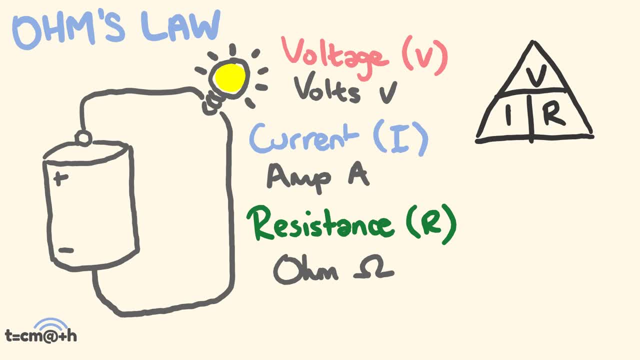 this saves you remembering a whole bunch of formulas. you have it all written there and all you really need to know is that voltage is equal to current multiplied by resistance. you draw up your triangle there and then you can start working out all sorts of things there, but, as you can see, voltage, current, resistance are totally related to one another. so let's do some. 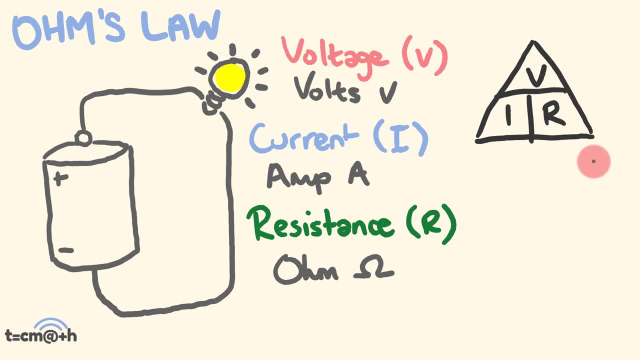 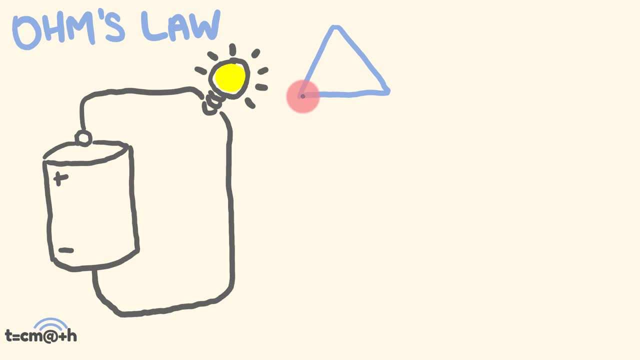 problems that you might encounter with ohms law. so i'll get rid of these to start off with and once again, i'll draw my ohms law triangle over here. okay, so always a good way to start. i'll keep it there and it's going to be. voltage is equal to the current multiplied by the resistance, so i have my 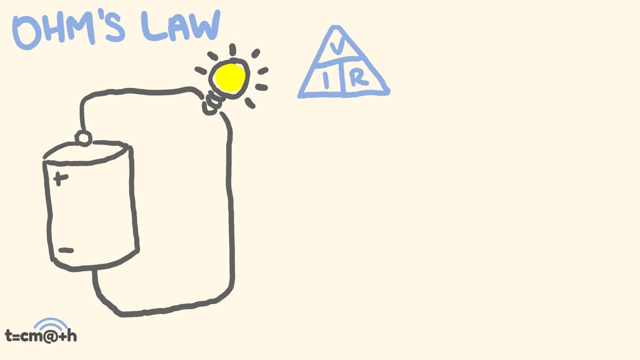 ohms law triangle. now let's go through and put some values into our particular diagram here. we'll get a bit fancy with our diagrams and do some proper diagrams in a minute. but let's start with this diagram and say, for instance, we had a six volt battery and then what we did is we got an. 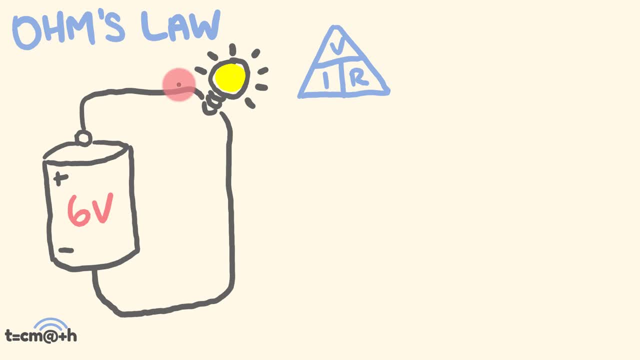 ammeter and we actually measured how much current is going through the wires here, and when we did that, we found out that we had a current of 1.5 amps. okay, i is equal to the current multiplied by the resistance, equal to 1.5 amps. and you know what i'm going to ask? i'm going to say, okay, well, what is the? 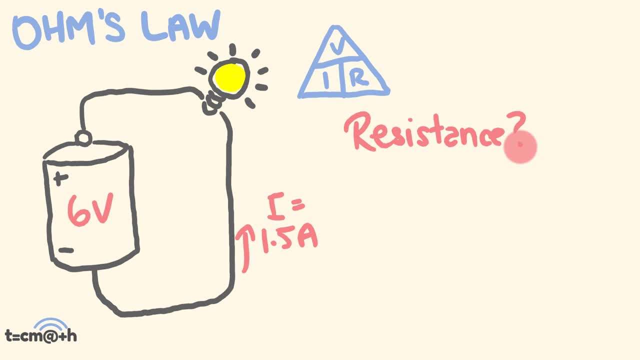 resistance equal to okay. so how much is resistance and how do we go through and work that out? well, it's pretty simple. we use our ohms law triangle. here we go the resistance, put our finger here and it's equal to the voltage over the current. so, equals the voltage over the current, all right. 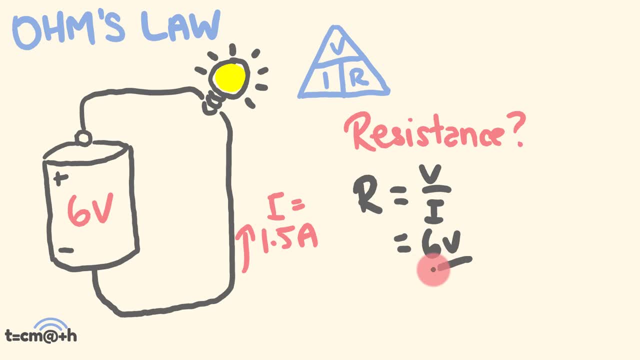 let's work this out. what's the voltage? well, you can see it's six volts and the current is 1.5 amps. six divided by 1.5, we get our answer. six divided by 1.5, we have four ohms is the resistance. 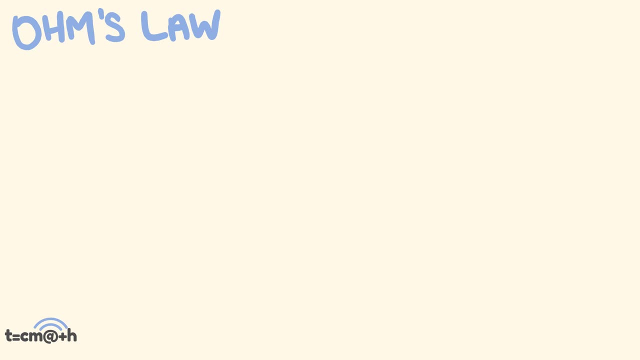 cool. well, let's do another one of these. so let's draw one more circuit up. i'm going to draw the proper schematics on this one this time. so first off, we have the power source, and this is how you draw these guys. we have the big line here, which is the positive, the little line here, which is 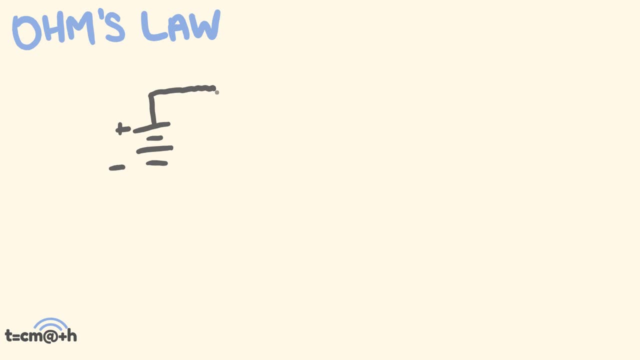 the negative. we have the wire coming off from that and we're going to show resistance. resistance is shown through this line here, the symbol here, and then the conductor goes all the way back around to the negative terminal there. let's put some values on our diagram, okay. so what we have? 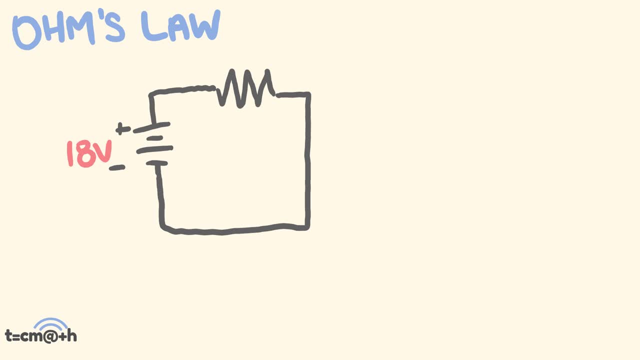 here is an 18 volt battery and we have a resistance that we know which is 24 ohms, and you know, we're going to be trying to work out. we're going to try and work out what the current is. so how do we go about doing this? well, first off, let's draw up our ohms law. 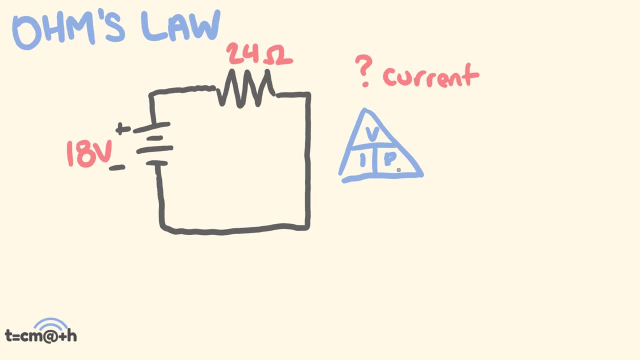 triangle. we have voltage equals current multiplied by resistance. we're trying to work out the current right here. so this is: the current is going to be equal to the voltage divided by the resistance. okay, so what have we got here? we have the voltage, which is 18 volts. we have the resistance, which is 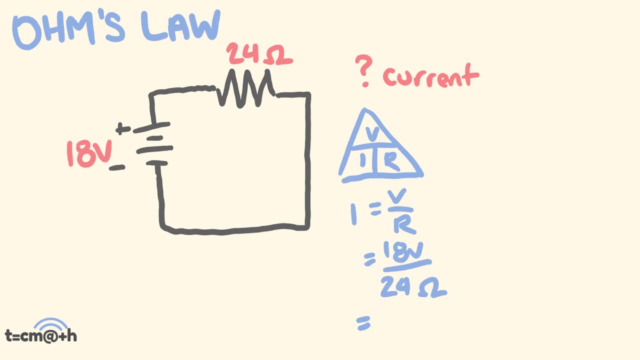 24 ohms, and we can work this out: 18 divided by 24, we get our answer, which is a current of 0.75 amps. okay, let's do some more of these. so i'm going to put up five more of these and do as many as you. 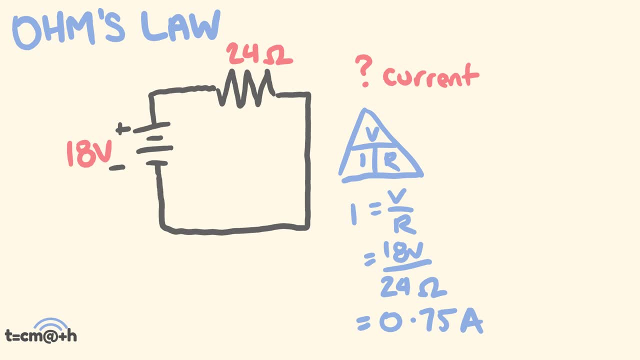 need to. it's well worth getting used to these, as they're needed in the next steps when we look at series and parallel circuits. by the way, if you like this video, let me know and subscribe. but here's some more questions. how many do i say i was going to do? we're going to do five more. 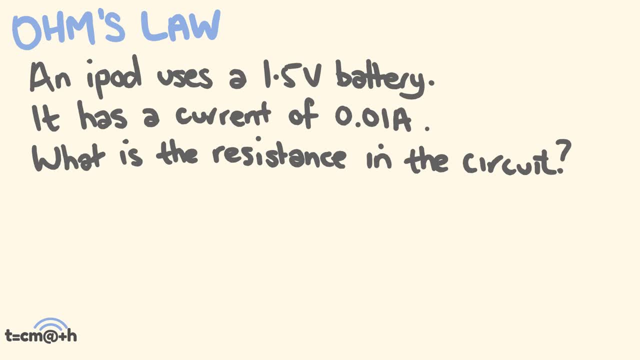 okay, the first of five questions. an ipod uses a 1.5 volt battery. it has a current of 0.01 amps. what is the resistance in the circuit? so you know how we're going to solve this. first off, we're going to draw up our ohms law triangle. that voltage is equal to current multiplied by. 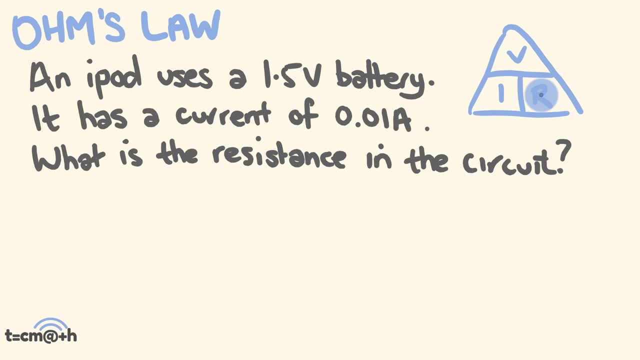 resistance and we're trying to work out the resistance. the resistance is equal to the voltage divided by the current. resistance equals voltage divided by the current, and this is going to be equal to the following: we have a voltage of 1.5- 1.5 volts and we have a current. 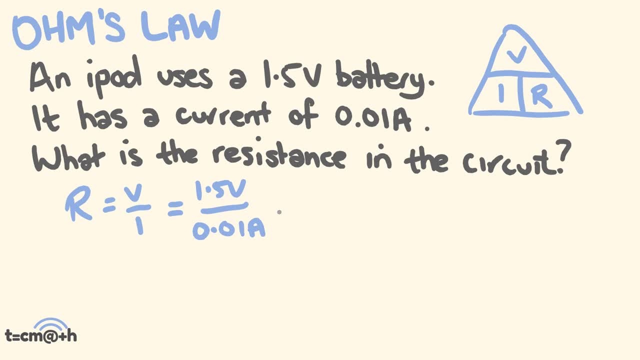 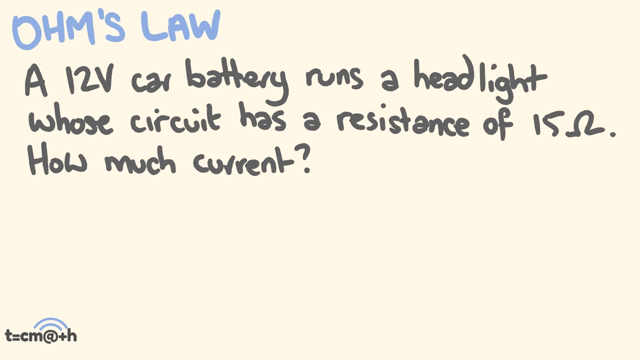 of 0.01 amps, nice and easy. 1.5 divided by 0.01, we get our answer here. we have a resistance of 150 ohms. nice and easy, cool. what about we do a second question? okay, our second question. a 12 volt car battery runs a headlight whose circuit has a resistance of 15 ohms. 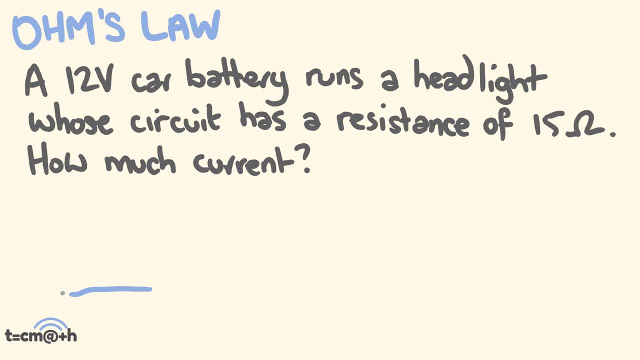 how much is the current we're talking about here? so what would i do first? well, draw my ohms law triangle up and i'm going to say: voltage equals current multiplied by resistance. we're trying to work out the current here. so current is equal to voltage divided by resistance. 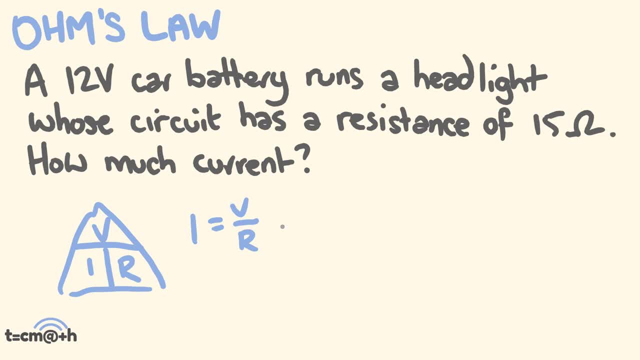 so current is equal to voltage divided by resistance, which is equal to the following: the voltage is 12 volts, we have the resistance, which is 15 ohms, and we're going to get an answer. it's going to be, in amps, 12 divided by 15.. we get our answer of zero. 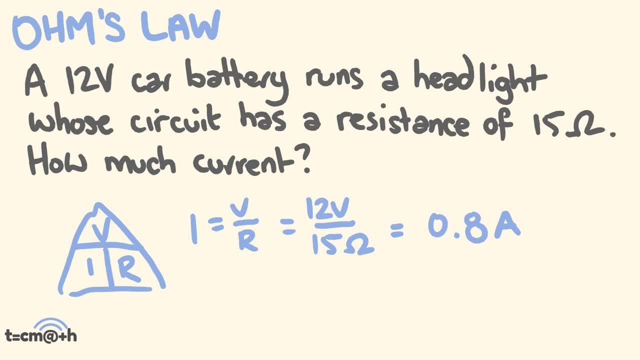 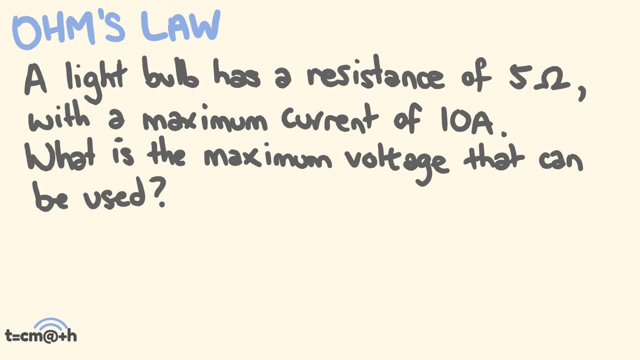 0.8 amps. the current is 0.8 amps. these are pretty easy, right, okay? third question: a light bulb has a resistance of 5 ohms with a maximum current of 10 amps. what is the maximum voltage that can be used? so, once again, let's put our ohms law triangle there. 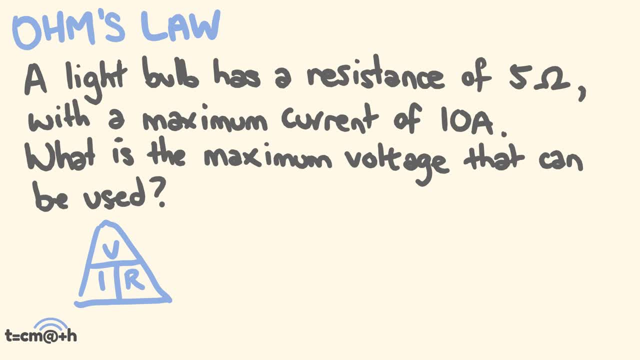 good practice, just get really used to it. voltage equals current multiplied by resistance. we're trying to work out voltage, so we're going to go. voltage equals current multiplied by resistance. nice and easy, we're just going to be multiplying. we have a current which is 10 amps. 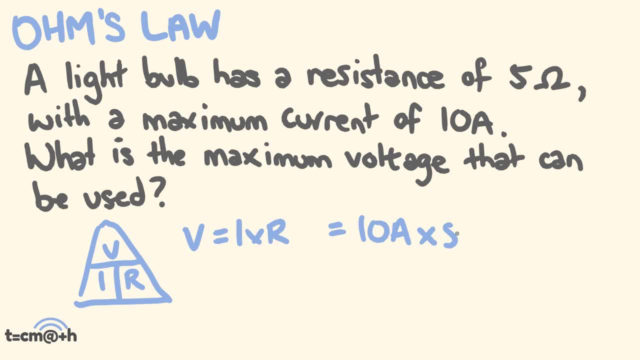 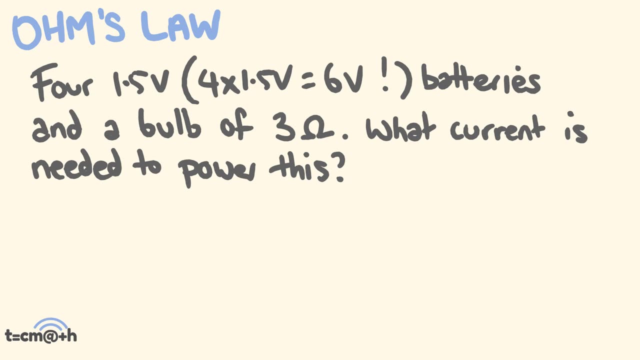 and we have a resistance which is 5 ohms. so 5 ohms and what do we get? 10 times 5, we have 50 volts. so the maximum voltage that can be used is 50 volts. all right, our fourth question- and you can see i've even stopped even writing proper questions these days- we have four: 1.5. 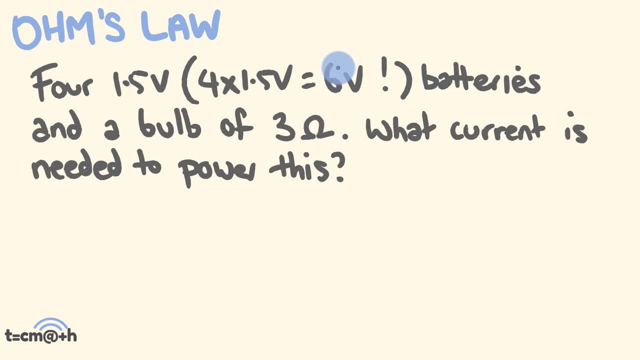 volt batteries, so four by 1.5, we have total of six volts running into this uh particular hour. I've got a bulb will be running in a major cell, the initial circuit, and we have the bulb which has a resistance of three ohms. okay, so what current is needed to power this? all right, so 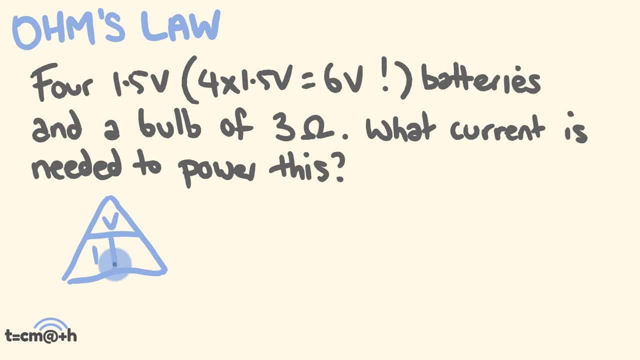 how do we go about doing this? all right, pretty simple. we draw up our triangle and we say that voltage is equal to current multiplied by resistance. we're trying to work out the current. so the current here is equal to the voltage divided by the resistance- six volts, and we have the resistance of three ohms and everything works out nice and easy. six. 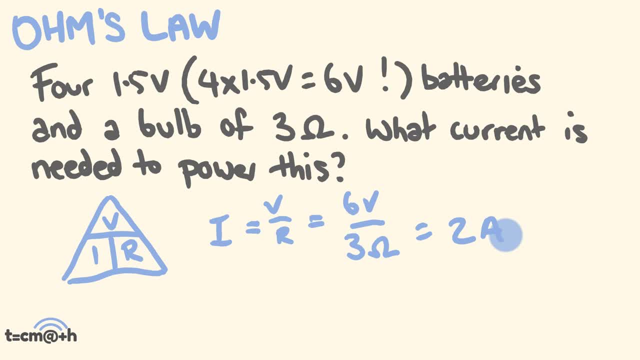 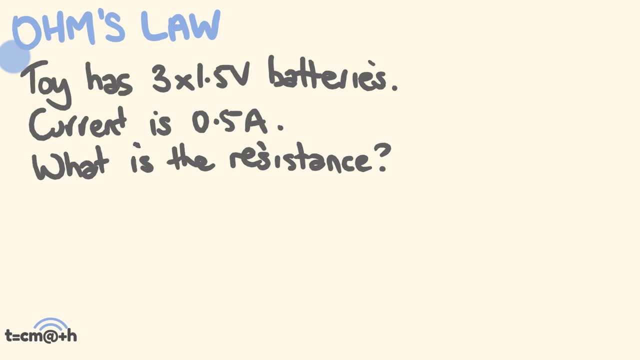 divided by three, we have two, two amps. so we have two amps of current running through that wire. all right, we're going to get to that last question. okay, final question. the toy has three 1.5 volt batteries. the current is 0.5 amps. what is the resistance? so let's draw this up first. we have 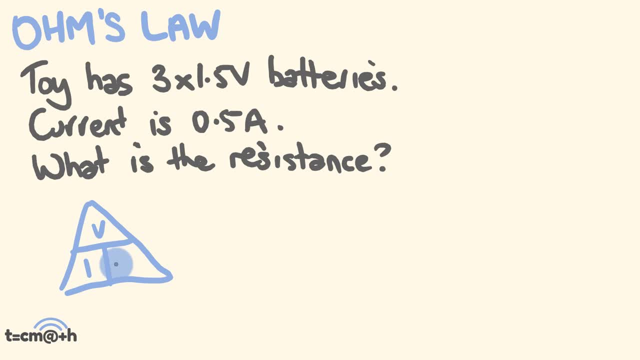 our ohms law triangle, voltage equals current times resistance. we're trying to work out the resistance, so the resistance here is going to equal the voltage divided by the current. easy, all right. so what's the voltage? it has three times 1.5 batteries. so three times 1.5 we have 4.5 volts. 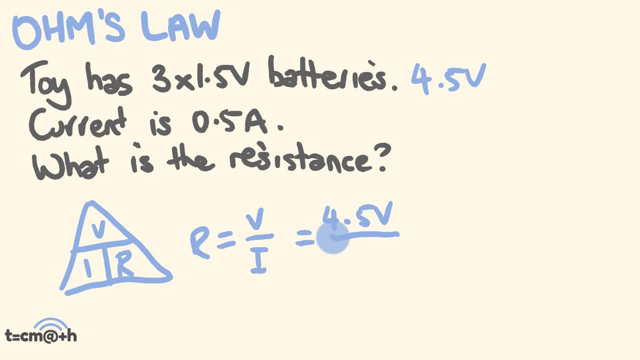 so let's put that in 4.5 volts and the current is 0.5 amps. let's put that in 0.5 amps: 4.5, 4.5, 4.5 divided by 0.5, that is going to equal 9, and the unit we use for resistance once again. 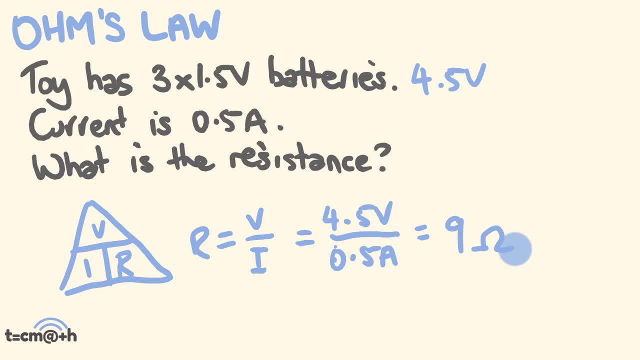 is ohms, because ohms is all about resistance. anyway, thank you for watching. there is an upcoming video where we're going to be looking at series and parallel circuits and it's really worth knowing your ohms law if we're going to get into those. anyway, i hope you like that video. like subscribe. you know the rest. thank you for watching. see you next time. bye.